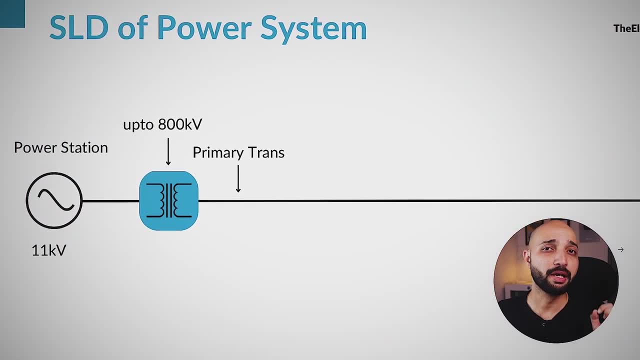 Now generating station will also be generated at a smaller voltage level around 11 kV. Now generating station will also be generated at a smaller voltage level around 11 kV. You will also have a connected substation called a generating substation, which is responsible. 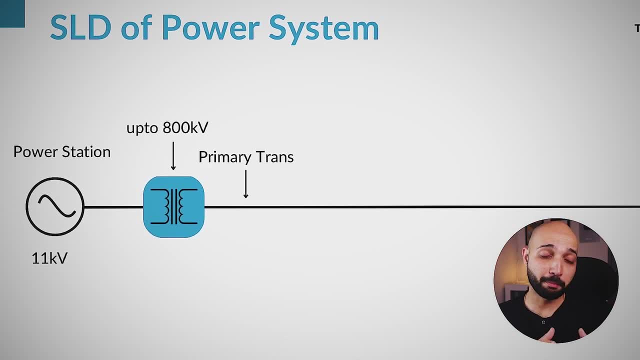 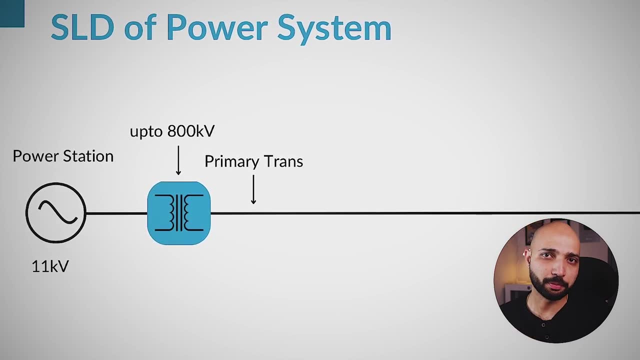 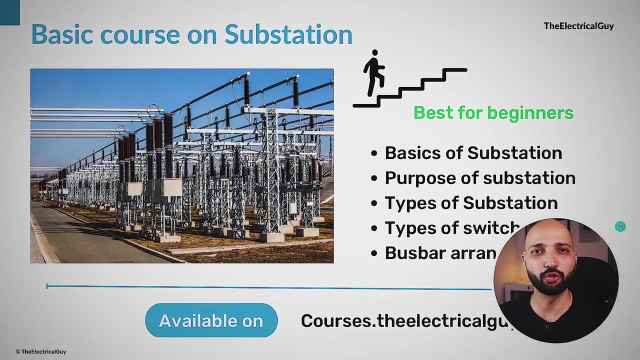 for stepping up the voltage. Now, what equipment are used in a substation? What is the circuit arrangement used in a substation That details are not shown here? The substation will have its own dedicated SLD. By the way, if you are interested, you can join my easiest course on substation. 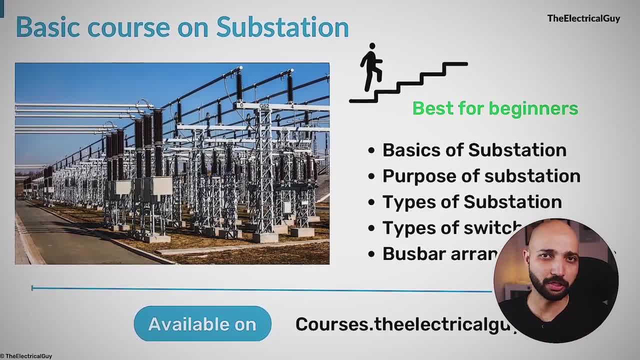 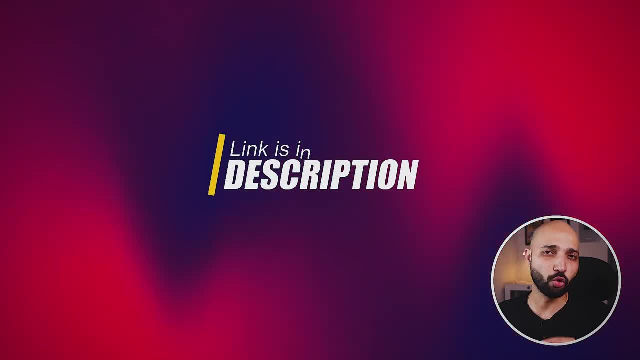 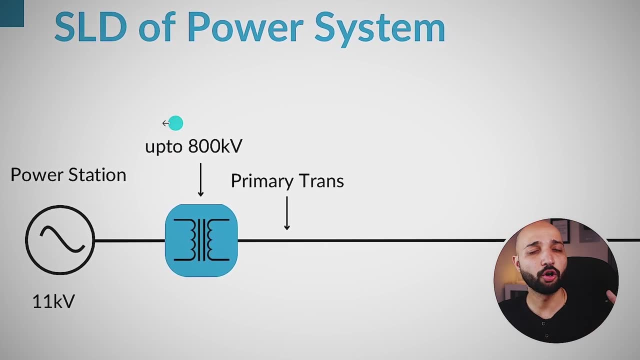 This would really help you if you are a beginner in the study of substation. It is available at coursestheelectricalguidein. link is also provided in the description. go and check it out now. this generating substation will step up a voltage to 145 or 245 or maybe 400 kv, or maybe. 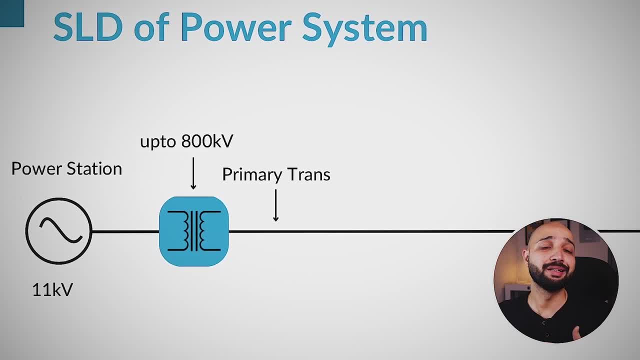 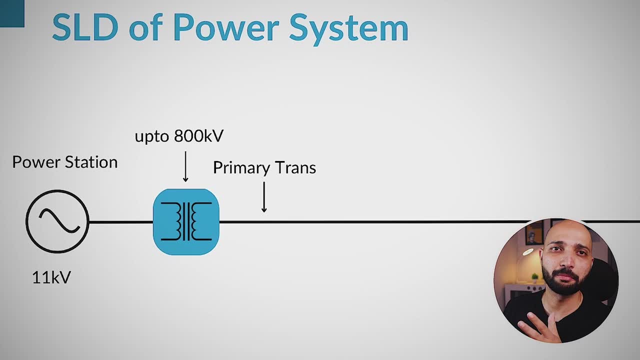 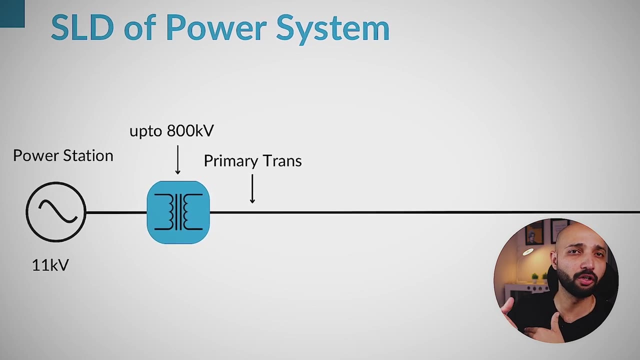 even 800 kv level. the voltage level depends upon the distance to which the electricity needs to be transmitted. higher the distance, higher will be the voltage level. for example, if the distance is, let's say, more than 200 kilometers, then transmitting the voltage maybe at 800 kv or 420 kv makes more sense. 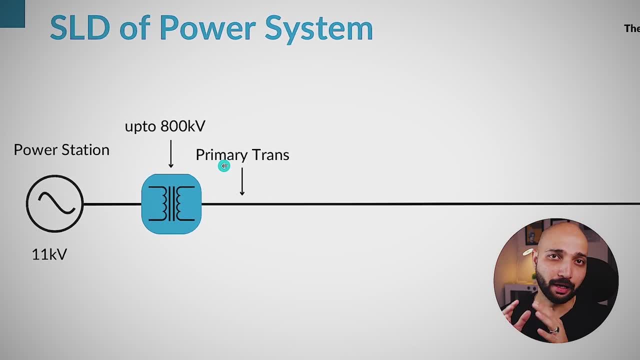 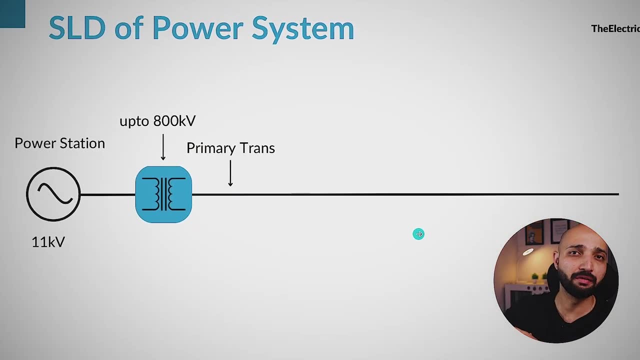 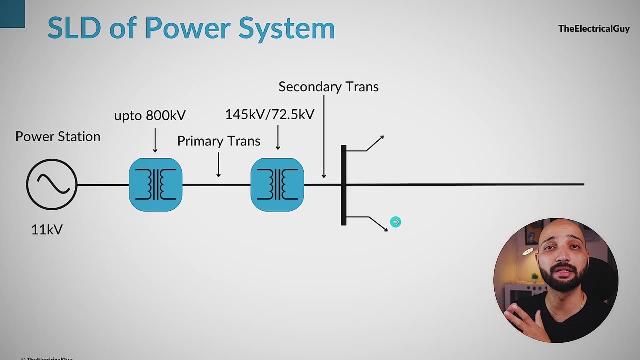 than transmitting it at 145 kv level, and this transmission level is called primary transmission. so voltage levels from 145 to 800 kv comes under the primary transmission. once the power is reached to the receiving substation, the power is then stepped down to the lower voltages. 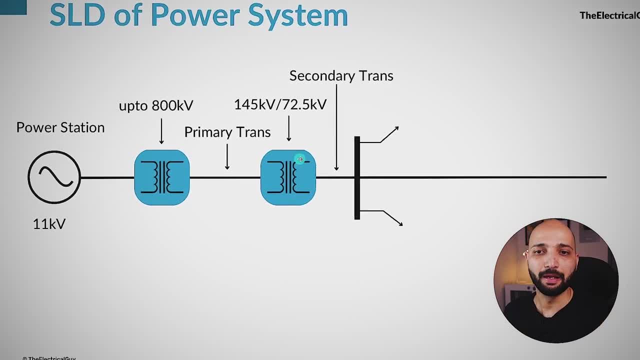 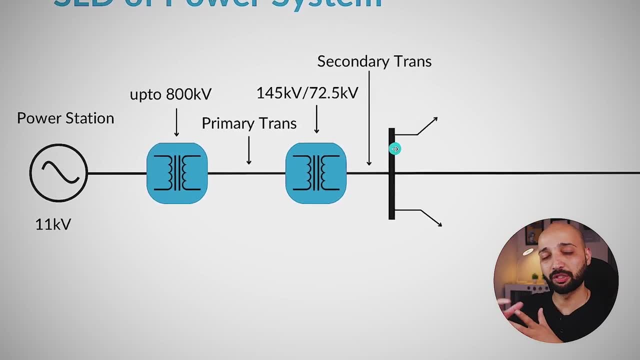 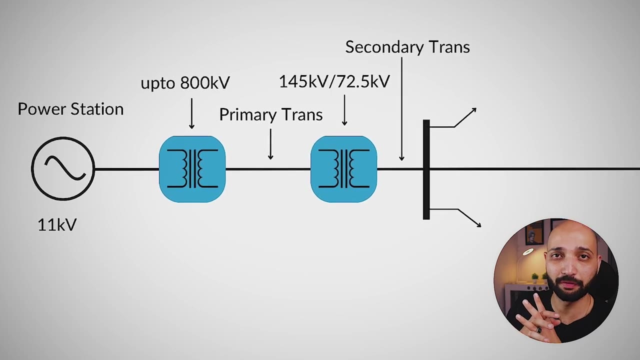 power will be stepped down to maybe, let's say, 72.5 kv, and this is the receiving station where the power is stepped down now, here. from here, the power can also be given to some of the ht consumer who needs to have, let's say directly, 145 kv in their factory or 72.5 kv in their factory. 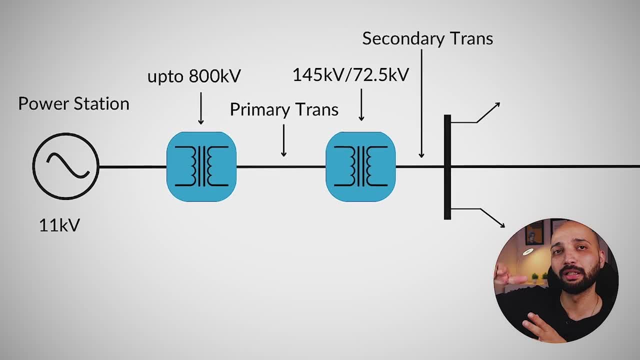 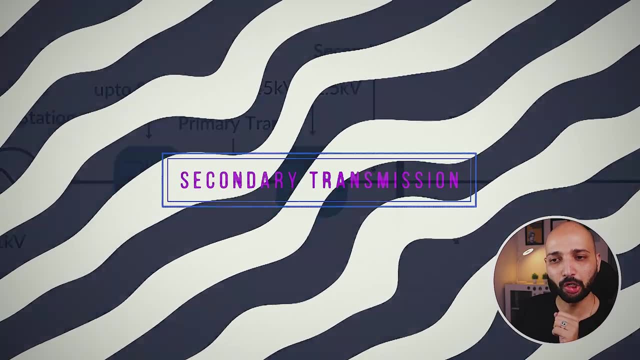 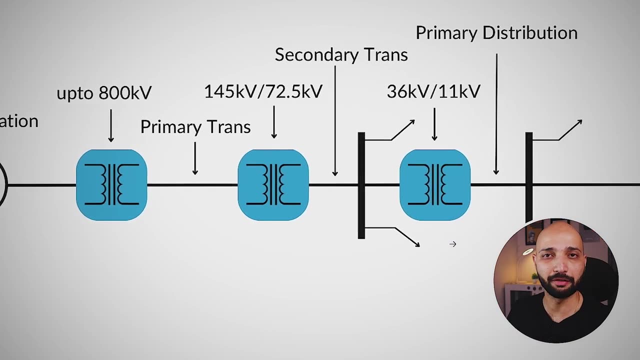 so from there they will build a step down substation and then they will take the power from there. so this phase is what we call as secondary transmission. now, moving on the secondary transmission, the power is again then stepped down to 36 kv or 11 kv now, after the 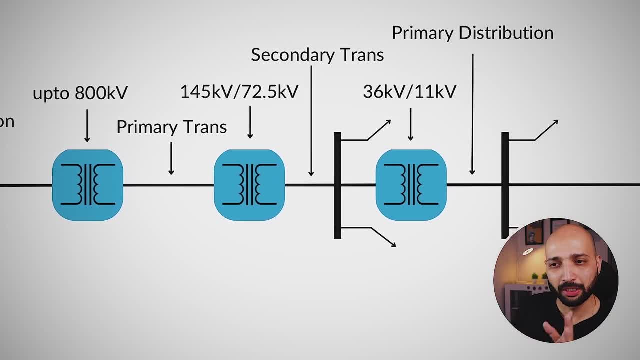 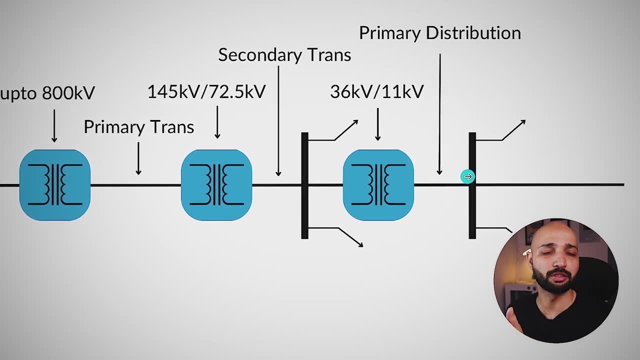 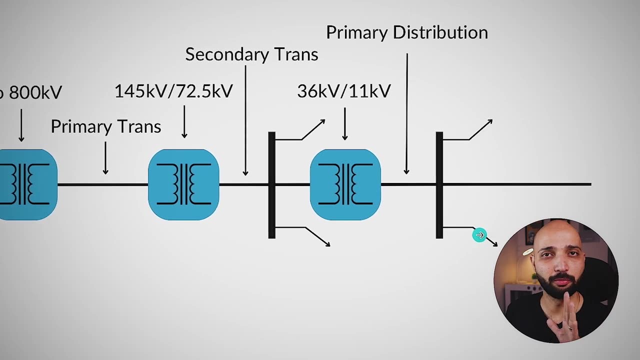 transmission we are entering into the distribution zone, so 36 kv or 11 kv is what we call as primary distribution. from here also the power can be given to the some of the consumers who needs to have 36 kv or 11 kv directly in their plant. so this is the primary distribution now.